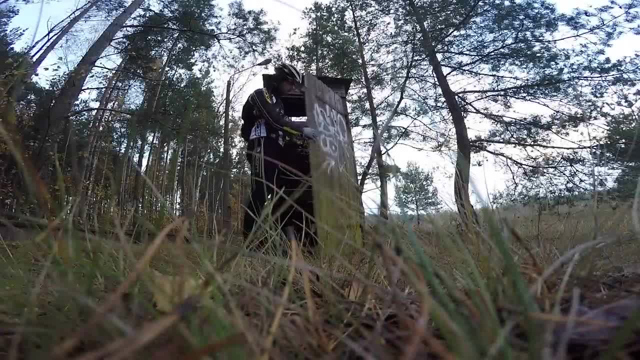 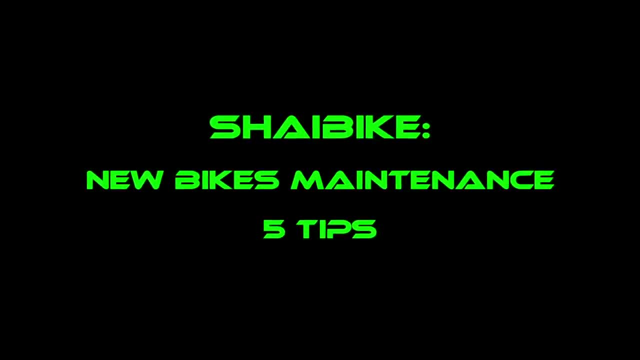 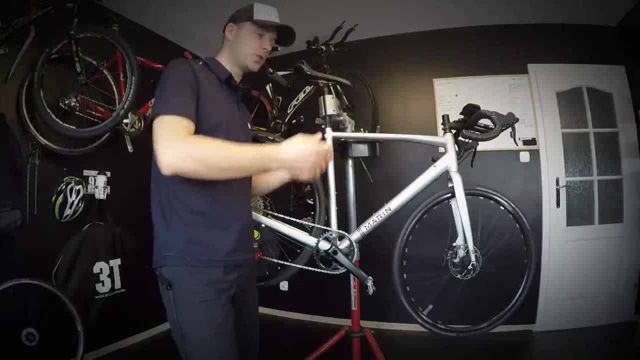 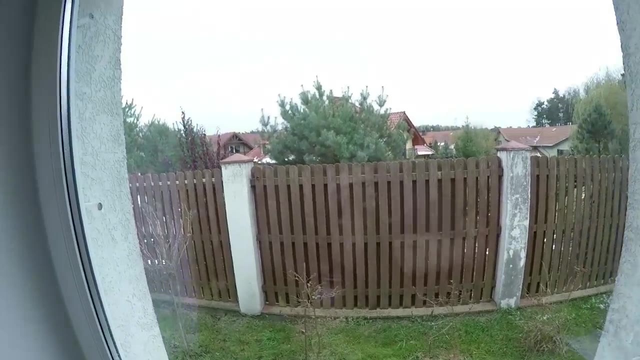 How are you doing, Sherbacks? I've been just wondering what's the weather like where you guys live, because here in Poland, I would say, the winter just came. you don't see maybe that much of a snow right now, but it's quite cold. so today. 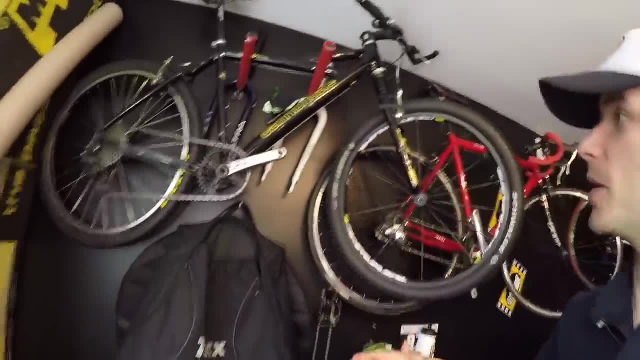 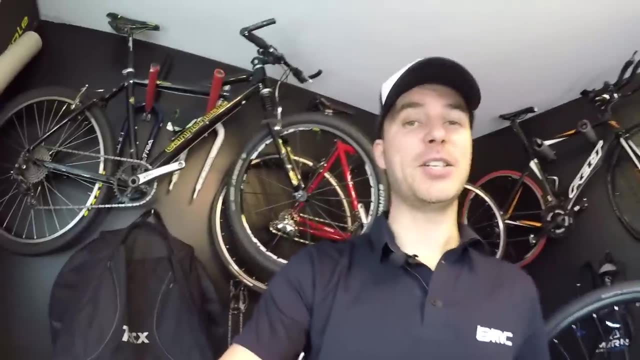 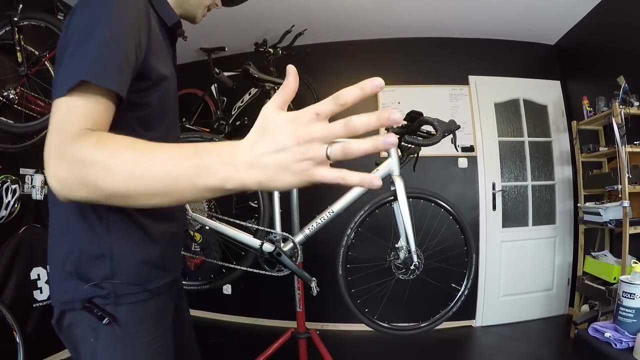 I'm spending more time in the studio doing some maintenance, like preparing killer for the winter. by the way, there is something new coming from Cannondale to my studio and it should arrive within two weeks. it will be so exciting, so stay tuned for that. but today we're talking about five maintenance things. 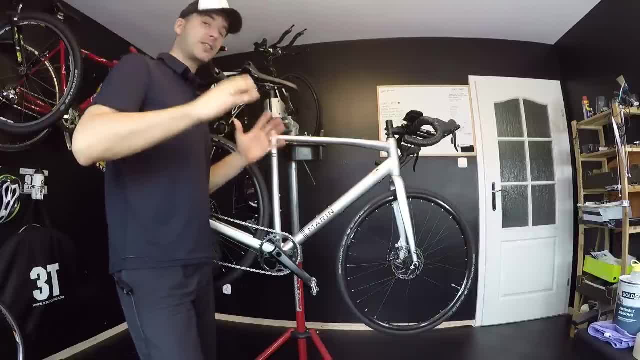 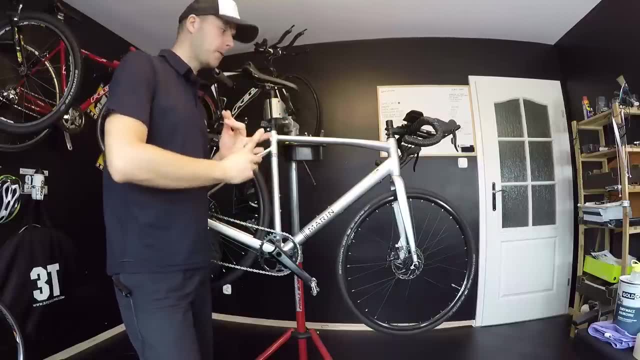 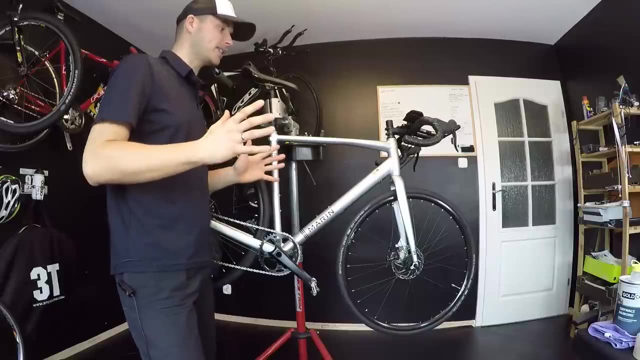 you should do with your new bikes. basically, I'm trying to tell you that if you purchase new bike, either in the store, like your local store, or online, it's not quite ready for writing and unfortunately, there's so many things that some manufacturers, or most of the manufacturers, don't care about. I'm going 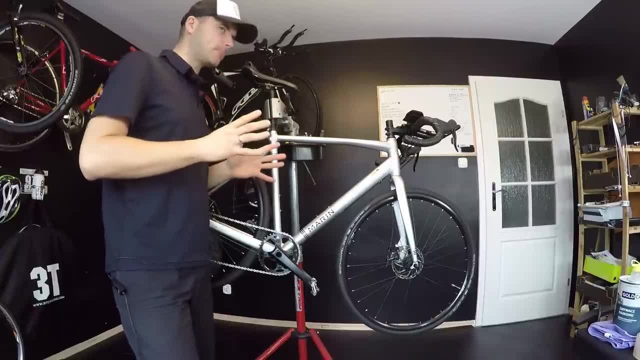 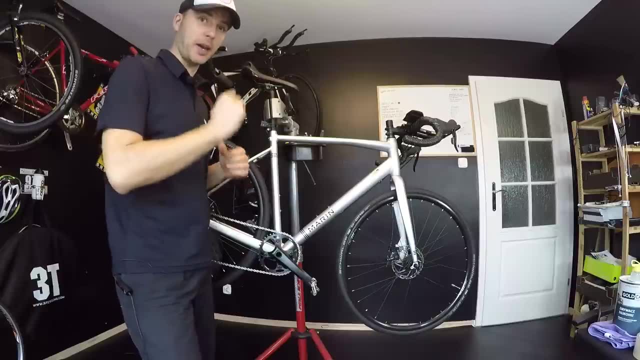 to point those out right now. I'm pretty sure that maybe 99% of you guys would have to do at least two of those things on your new bikes. shall we start? all right, let's start here. we have a new marine gestalt. by the way, I'm not. 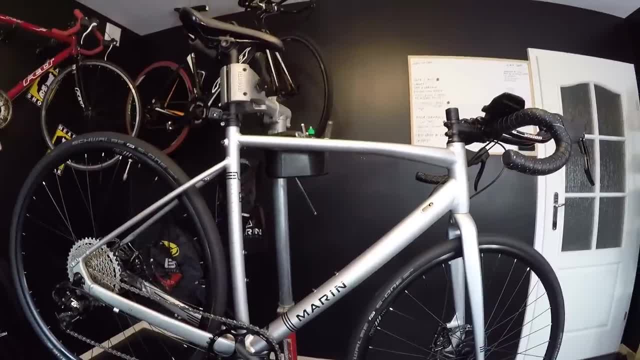 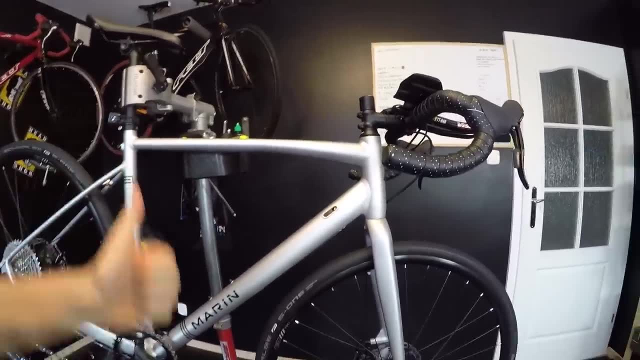 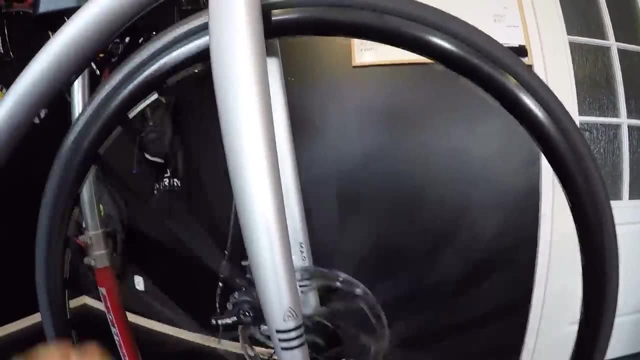 picking on this bike. what I'm talking about in this episode is just my experience from purchasing different bicycles, but let's start with the first thing, and that's the wheels. when you purchase the bike, you should definitely, definitely check out whether the wheels are true, because, as you can see, this one 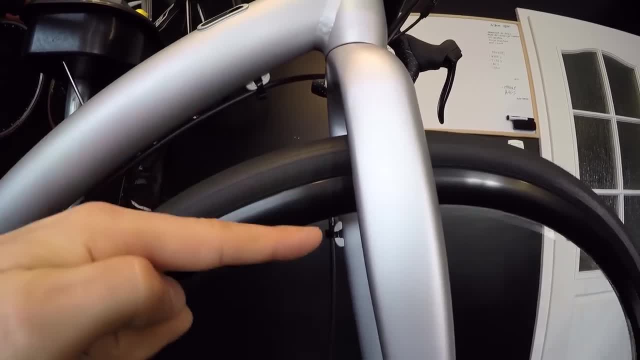 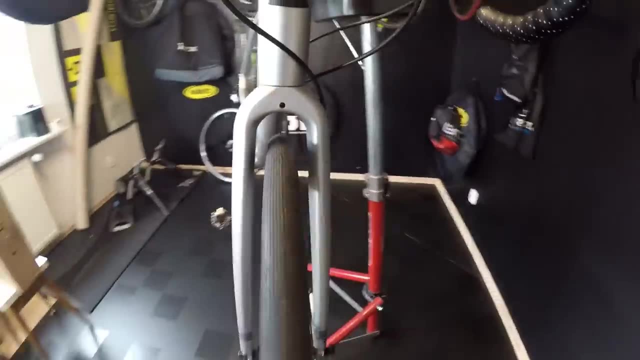 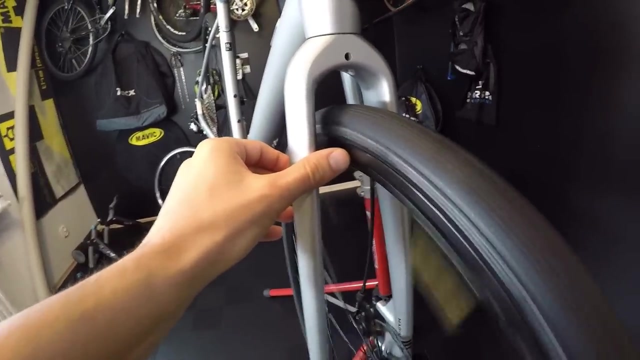 isn't quite true. you can see the rim moving up and down. that's not really good. and also when you look from like from the back or from the from the front of the bike, you can also check out how true the rim is. and this one moves also from side to. 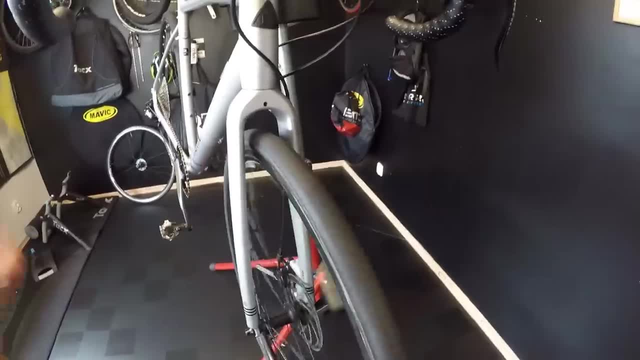 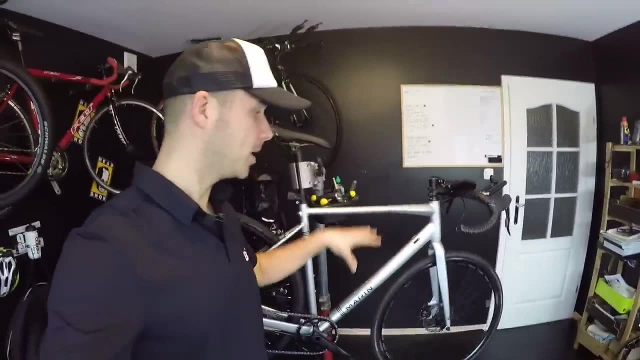 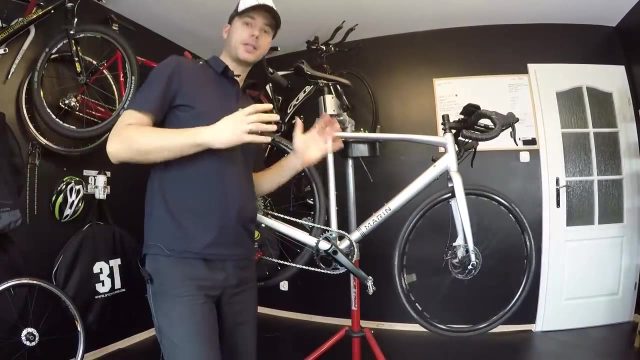 side for about one or two millimeters. so that's one thing that you could actually and you should actually go back with the bike to the store and say, hey, please, true, my wheels- because all the new wheels- doesn't matter how expensive or your bicycle was- should be hundred percent true. and also, after a couple of 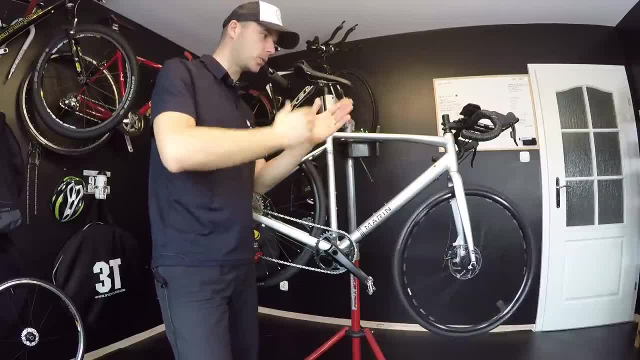 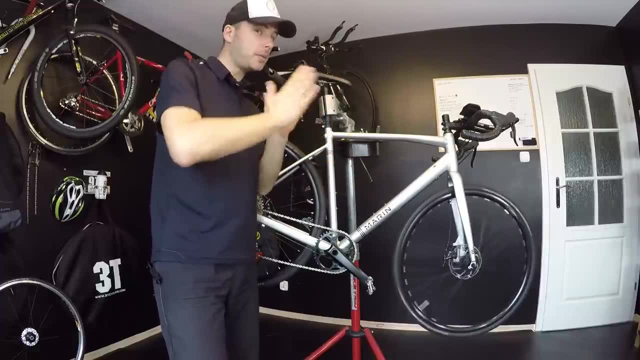 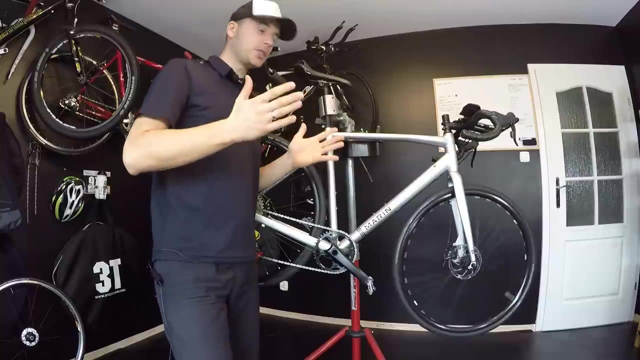 rides. those spokes will just find their place in the whole structure of the wheel. The wheel can come a little bit out of true? so then you should do the maintenance like truing the wheel. Of course, if you purchase the bike online, it's not really cost effective to be sending those. 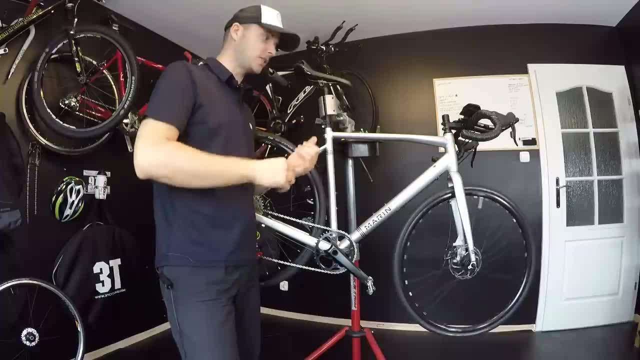 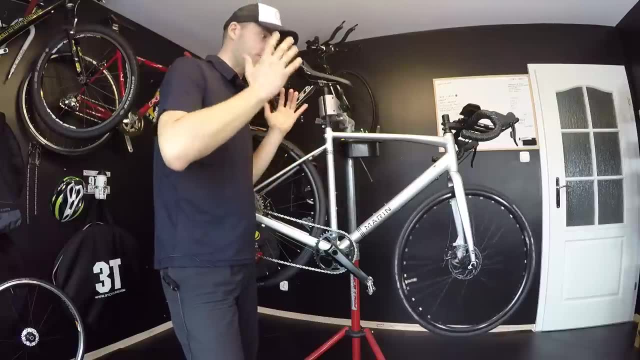 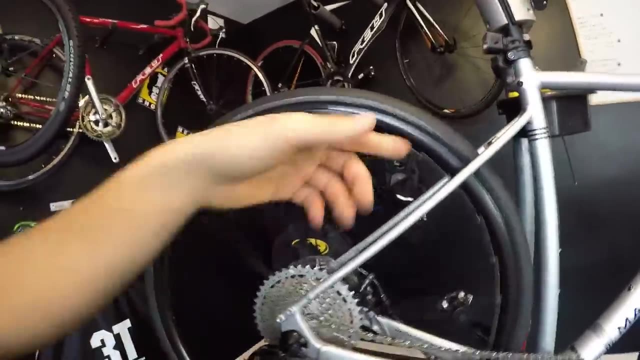 wheels back to the store just to make some little adjustments. If you can do it for yourself, do it. If you can't go to your local store and just ask people to do it for you, because many wheels will not be hundred percent true, I would say up to one millimeter is okay. This one is okay, up and down, but going. 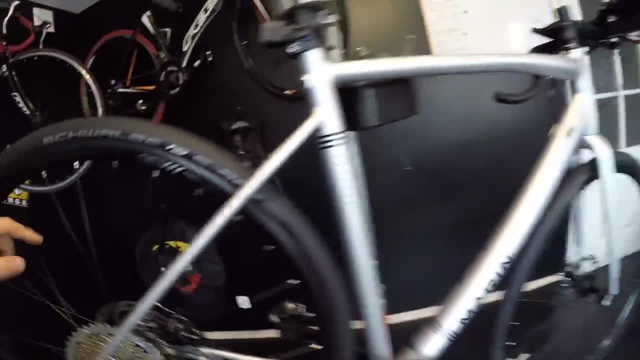 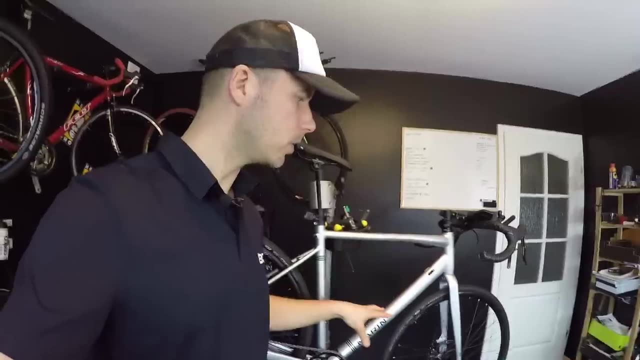 just a little bit from side to side. The rear one is better, The front one needs some adjustments. It's not like a bad wheel, It just needs adjustments. I would say also that if you purchase the bike with some stock wheels- Stock wheels I mean, if you purchase like- 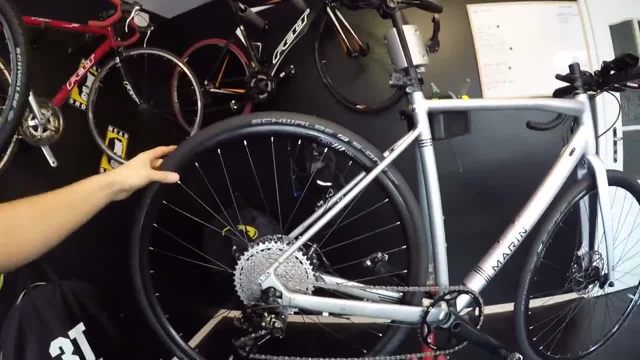 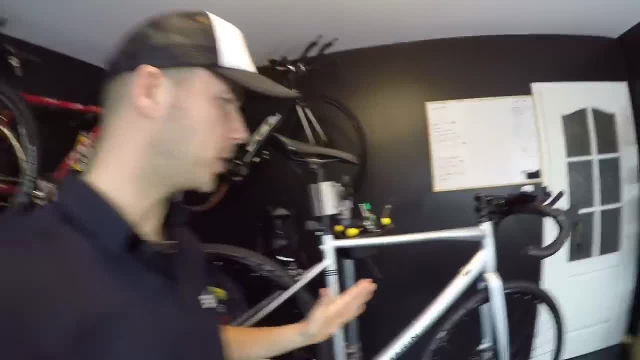 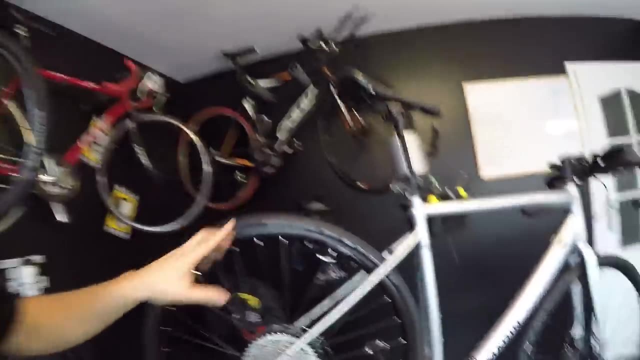 Marin Trek Giant Cannondale on Mavic wheels, on Campagnolo wheels, on Fulcrum wheels. These would normally be very good, but if you purchase the bike which just puts their stickers onto some cheap wheels, usually they really save time by. 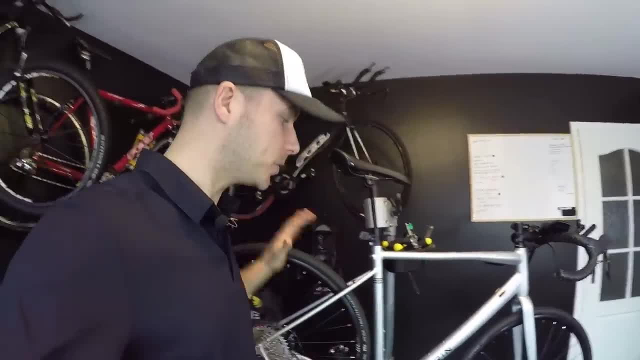 lacing those wheels. If you purchase the bike which just puts their stickers onto some cheap wheels, usually they really save time by lacing those wheels like super quickly in the factory and those just need adjustment. Those could be just fine, good wheels, but need adjustments. So that would be first. 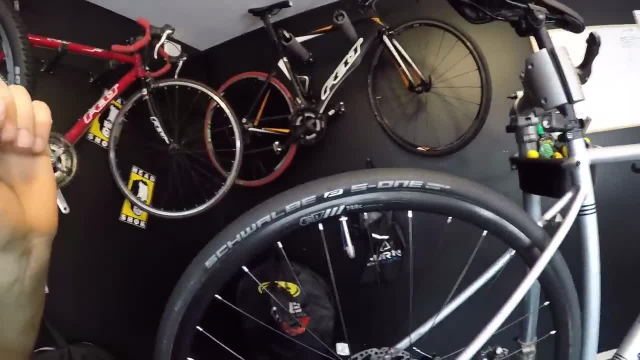 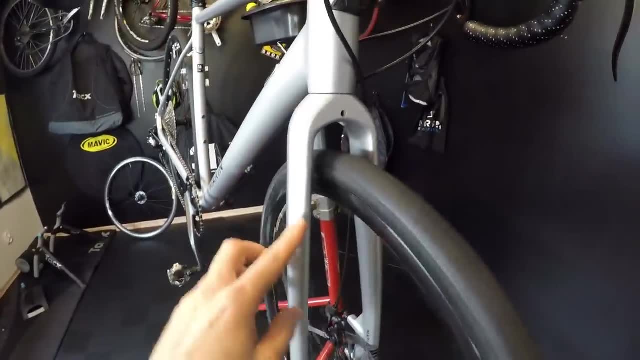 thing. The second one is the tires, because also, when you look at the tires, sometimes- and sometimes quite often- you may find out that the rim is okay, but the tire is moving either from side to side or up and down. If you've seen any of the movies showing how this wheel works- it's okay, Two wheels are okay- Then if you see any of the movies showing how this wheel works. it is okay, It's okay to use these low resistors power in one position, stick one wheel where never the other road unaided. The rim's okay. open the other one, put the other one on neutral, peppered it and remove it in single bilge trash. 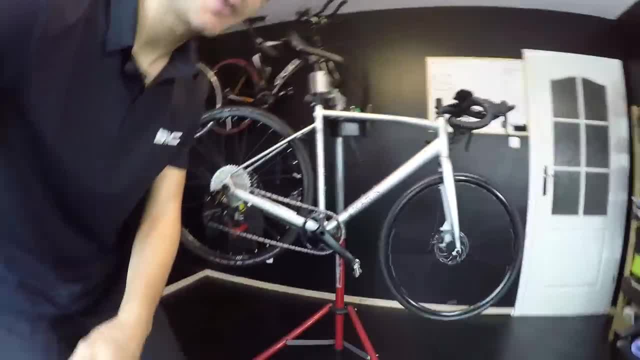 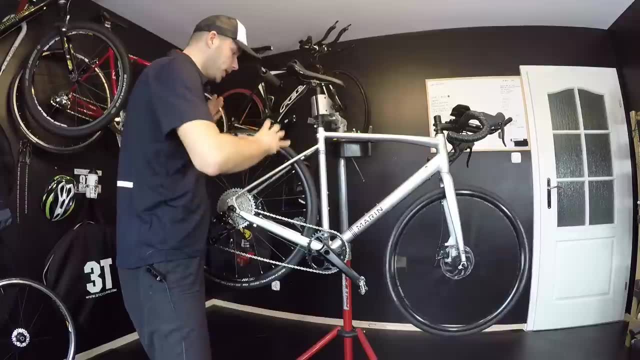 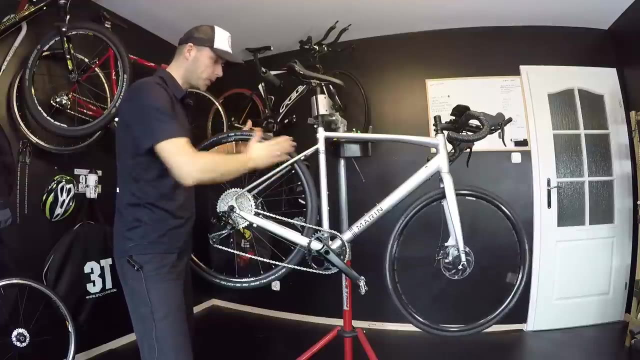 the movies showing how those, those guys working in the factories, like in taiwan- this one was made in indonesia- how do they actually put the inner tube into the wheel and then pump it? it's like 10 seconds. they just put the inner tube, they lock the tire and then, by using some pressure, they just 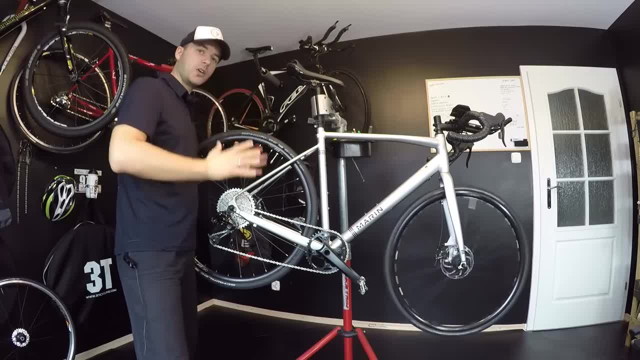 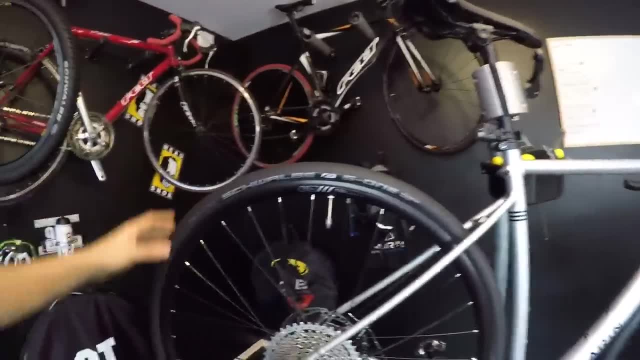 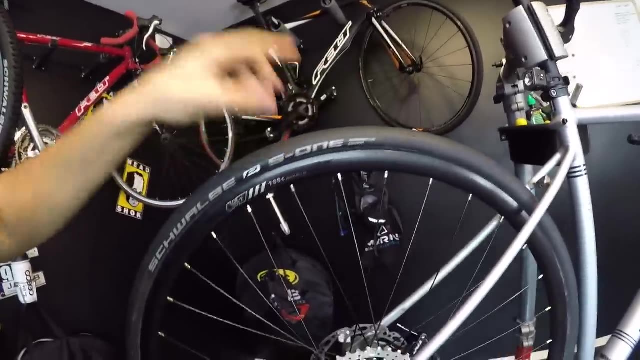 pump it up all at once, which we never should do like that, because when we pump the wheel- you can check out my other episode about it- we should pump first very, very little and then, um, try to help the tire to find its place in the rim and then pump into the full pressure that you really 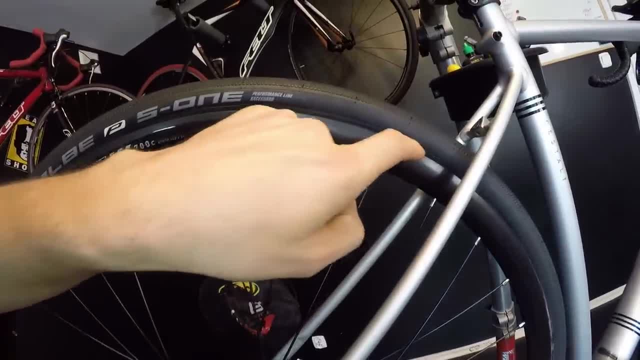 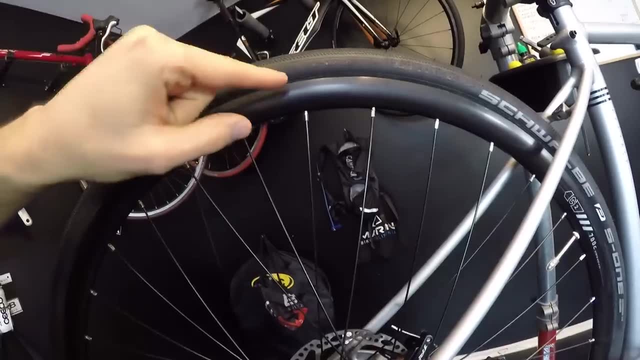 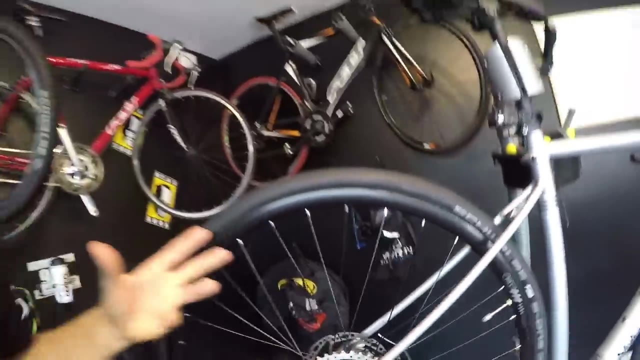 want to have on your bike so you can see the line or the marking here on the side of the, on the sidewall of the tire, and the distance between this mark or line and the rim should be always- even now some tires also are- are just lousy and not really true, but you should. what? 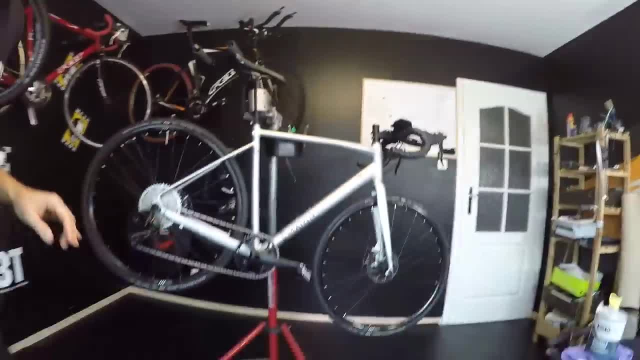 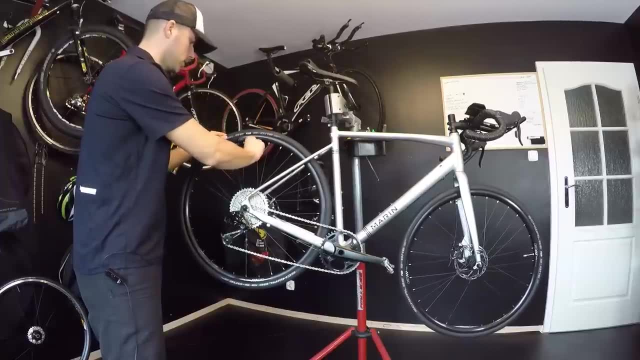 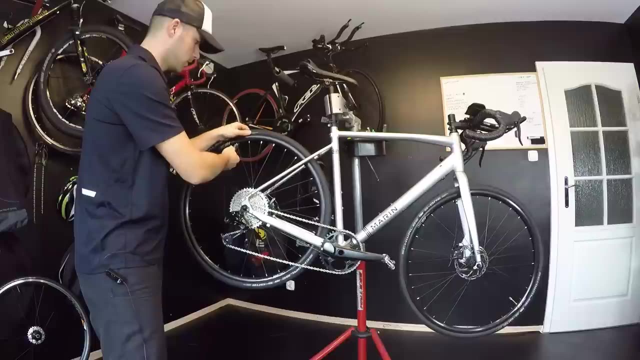 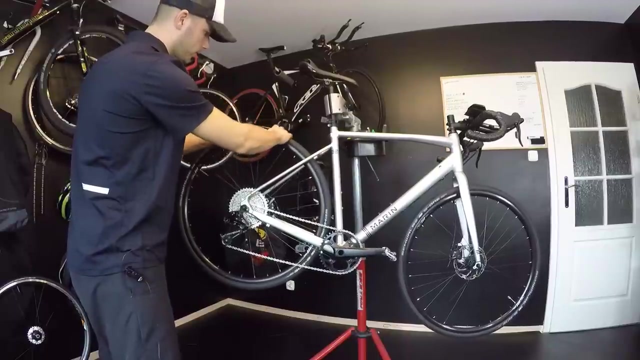 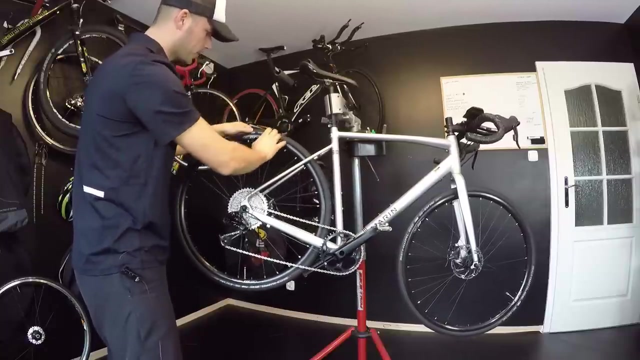 you should do with your new bike is to let me just show you very, very quickly: let out some of the air from the tire, okay, and then by pushing the sidewalls from both sides with our hands, we are helping the tire to actually fit into the walls of the rim. so you should have as little. 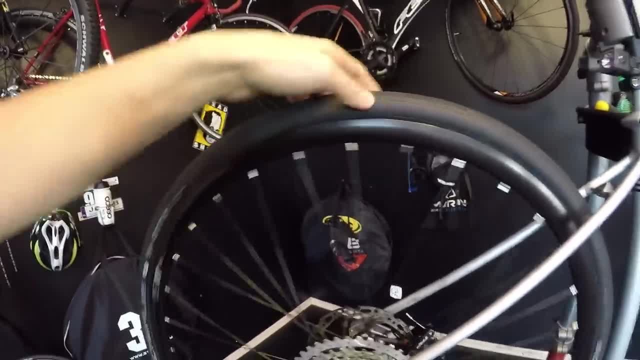 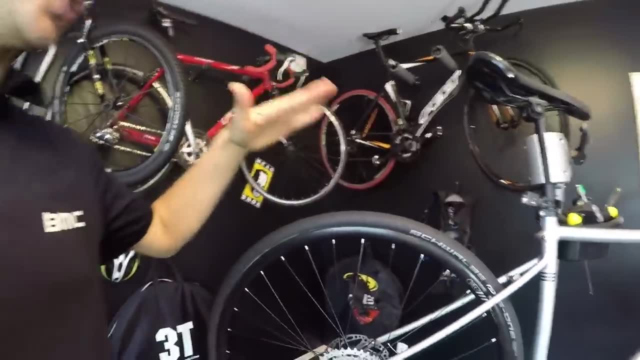 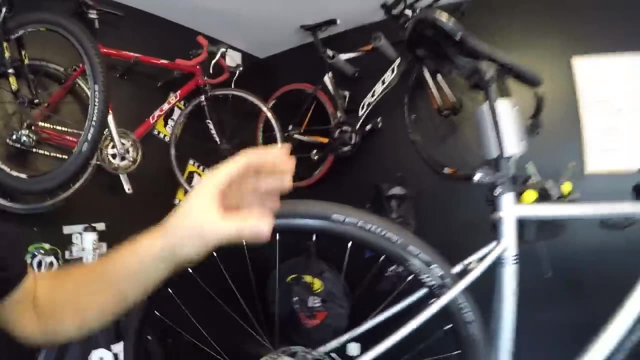 air, as it will just help you to do. do this so you can actually move around the tire in the wheel, then you can ride it. why is it important? of course you want to have true wheel and true tire, but also, quite often the the bead of the tire can kind of bite the inner tube if it's being done too quickly. 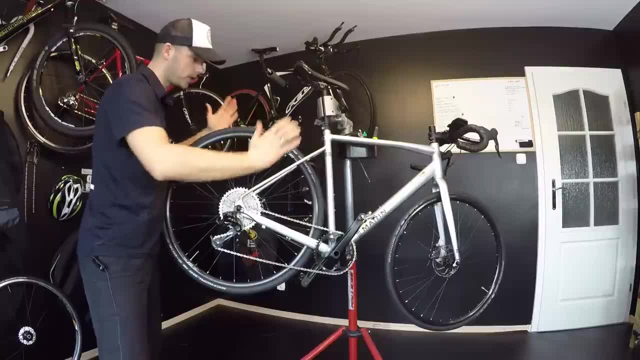 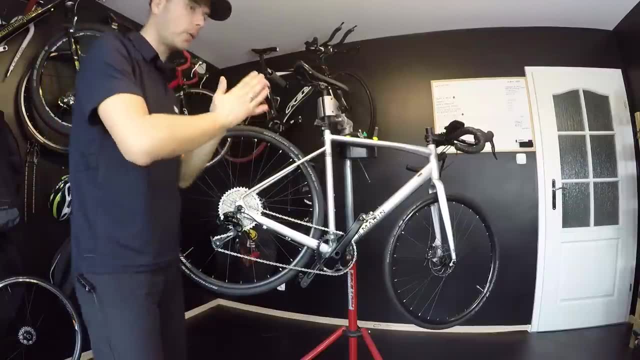 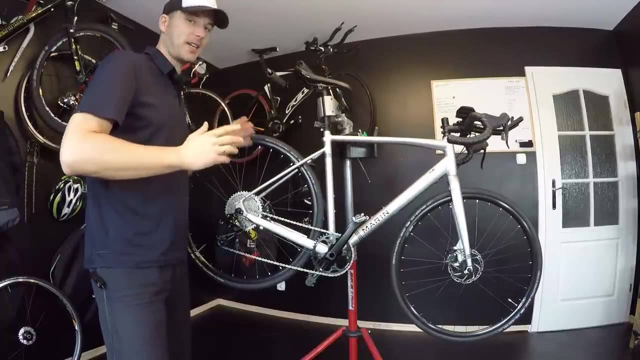 because if you put the inner tube into the tire, then you lock the bead and you pump it up just all at once. the the inner tube can always go just a little bit under the bead and then you just lose the inner tube and manufacturers just don't care about your inner tubes. that was also my experience. 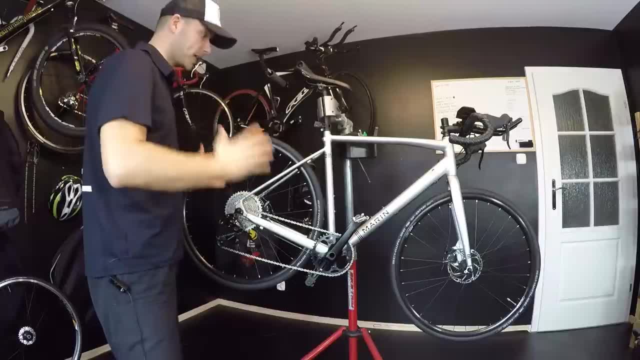 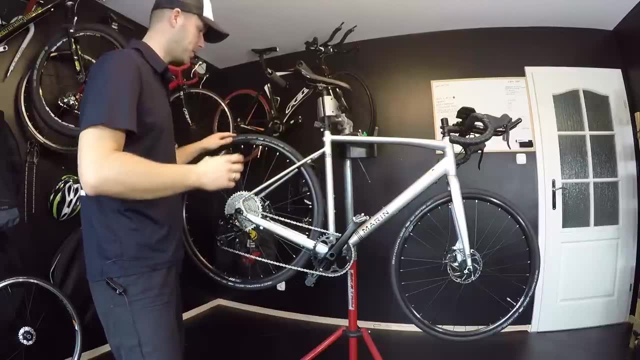 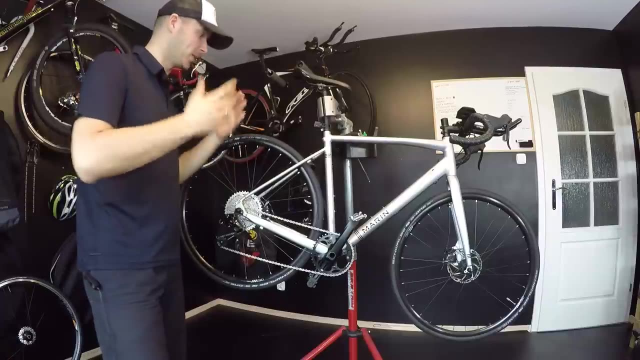 with Cannondale, my just beloved brand. so be careful of that if you don't mind. you know, losing maybe five or ten minutes to do that, you can save money for the inner tube or just save yourself by just, you know, puncturing somewhere in the middle of nowhere. so checking the how true your. 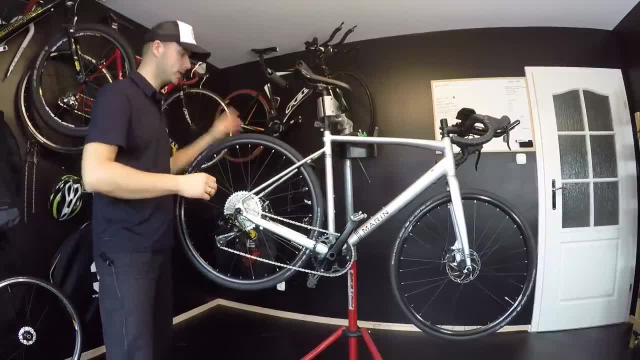 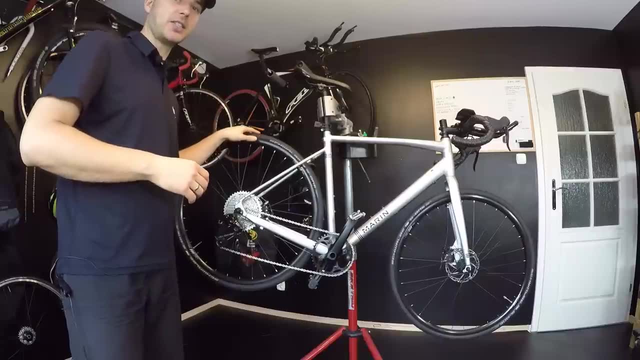 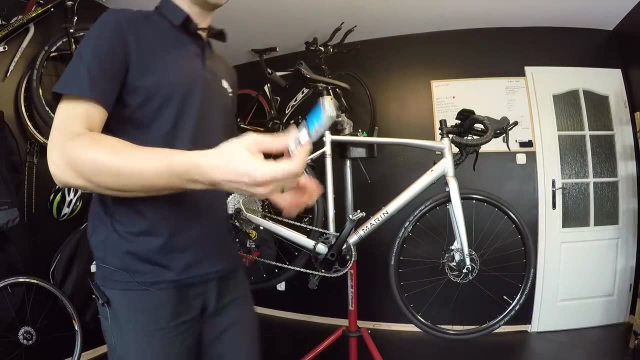 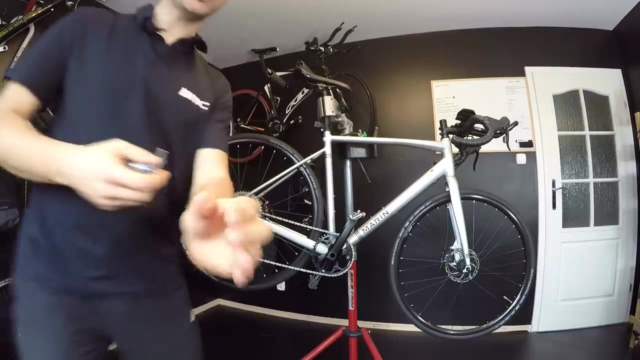 wheels are and adjusting it, just truing your wheels. second, checking how well the inner tube and the tire installation is on your bike is really important. then the third thing: it's also your safety. you just grab some multi-tool and check out all those bolts, all the bolts in the bike. so you just want to check out how well those are those tightened. so 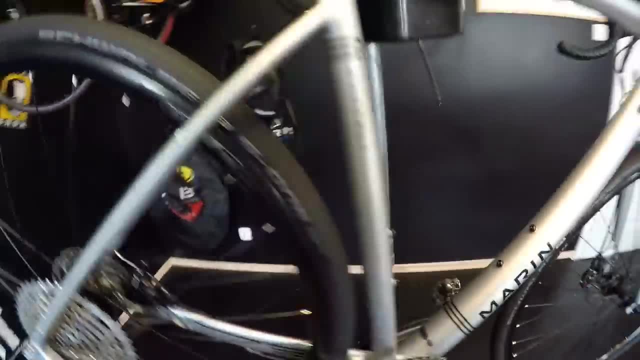 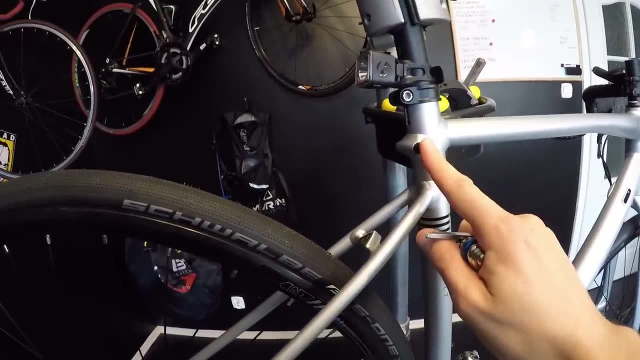 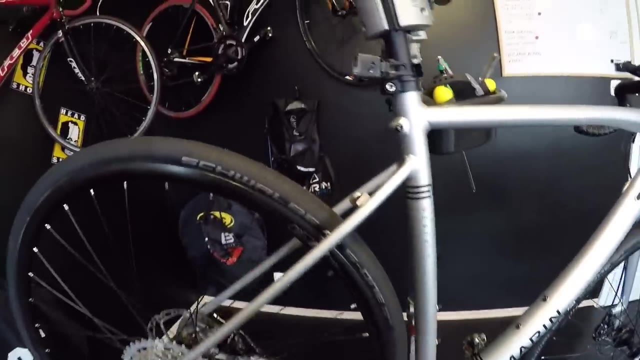 these bolts, like for the bottle cages. you just don't want to lose those. by the way, that was the case with this bolt here on the other side. it was almost lost when i went for the first ride. so check out if the bolts are just tightened well enough. i'm not saying that you should be tightening those. 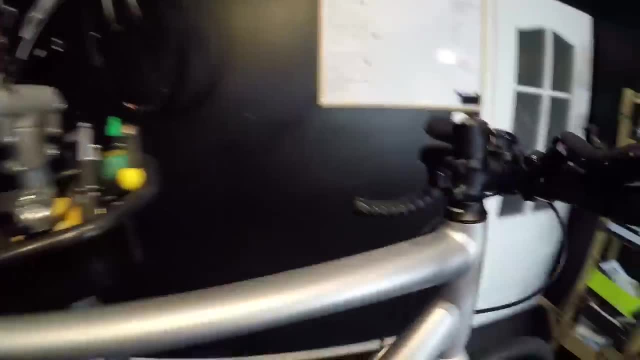 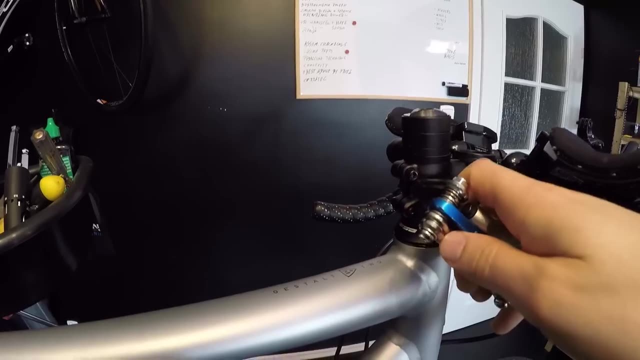 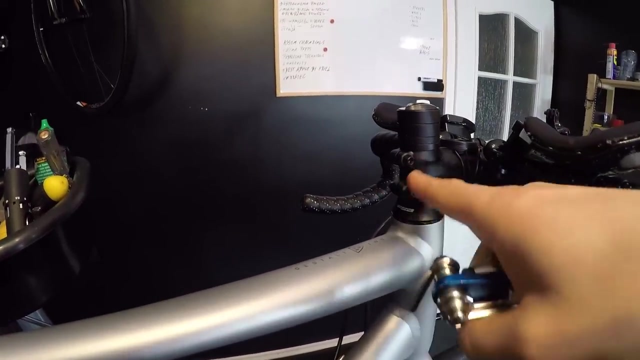 just check out whether these are not loose. important thing: you never mess up with this bolt from the headset when these two on the stem are tightened, so i would recommend to do that. so i would not just touch even this one, but always check out whether these bolts mounting. 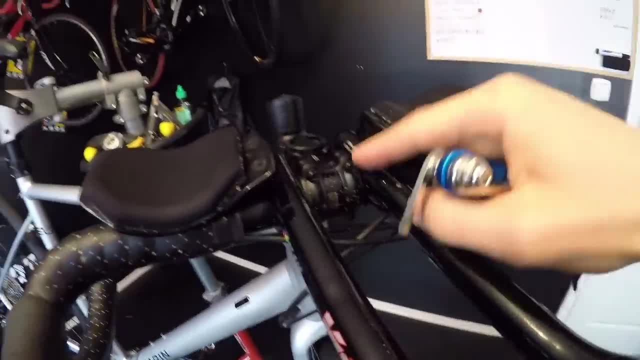 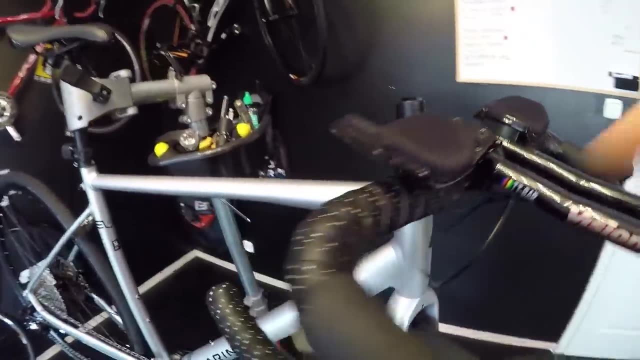 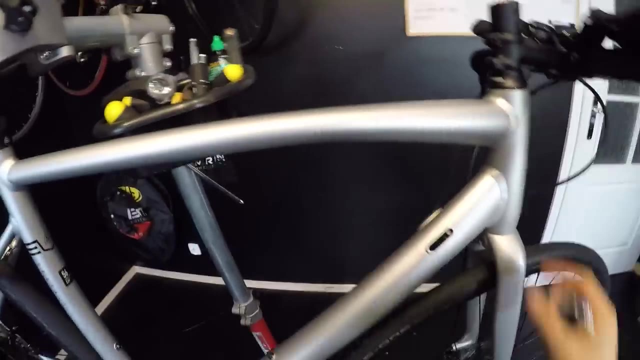 our stem are tightened and also the bolts that are tightening the handlebar to the stem. so just check it out. okay, it's not loose, loosen it's. it's fine and leave it. don't mess up. mess up with this one. um, when you will feel that you have some play in the headset, then you have to unscrew these and 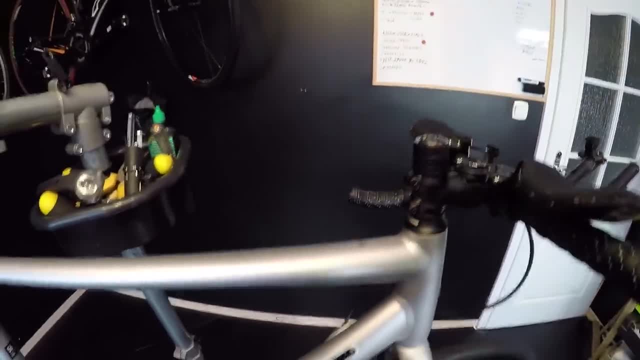 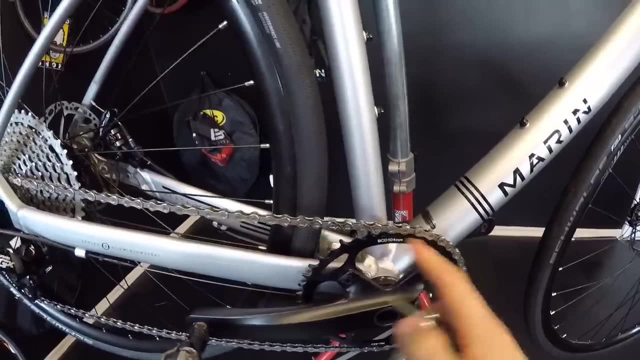 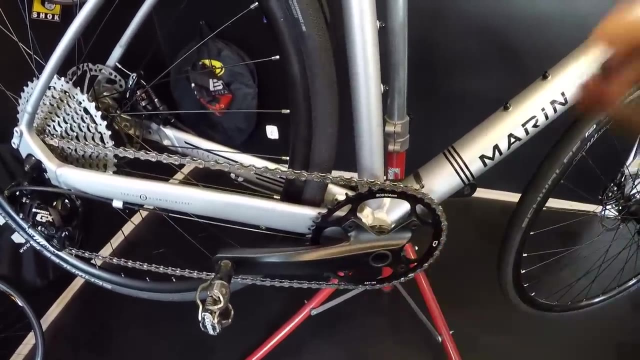 adjust the play with the with this bolt. i also made another episode on that very important thing: check out the bolts that are mounting your your crankset or chainrings. this can cause also some some creaking, some noise, if it's not done well. this bolt was quite loosened. 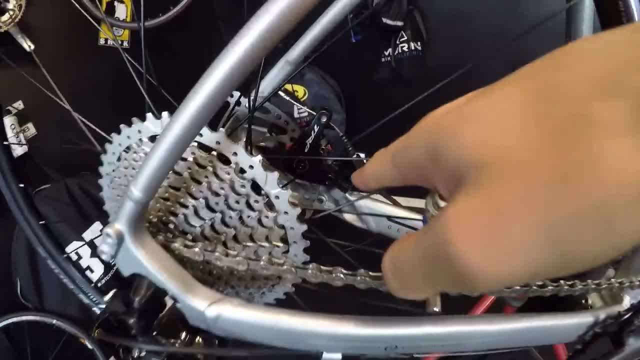 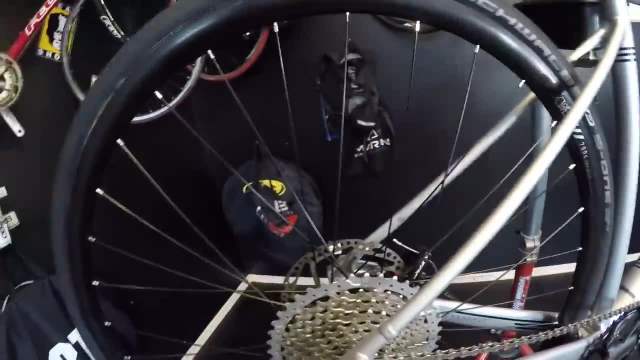 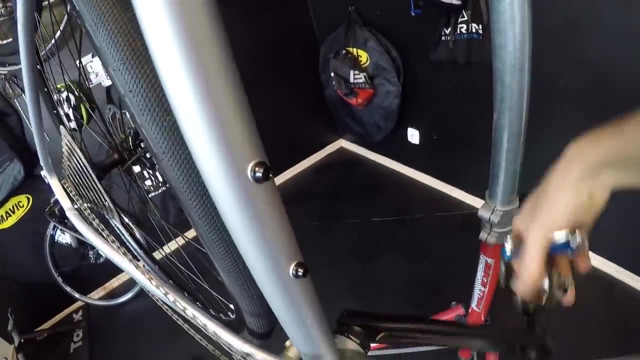 on this bike, by the way, and also the bolts on the other side that are assembling or um the the upper to the frame. just check it out. they should not be loosened. so another bolt is also here on the other side, um tightening the crank arm. unfortunately, you will find out quite often. 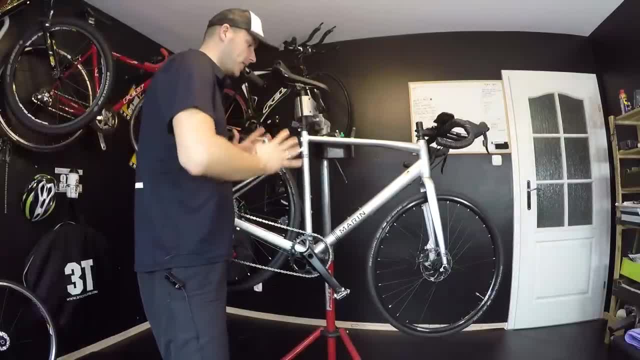 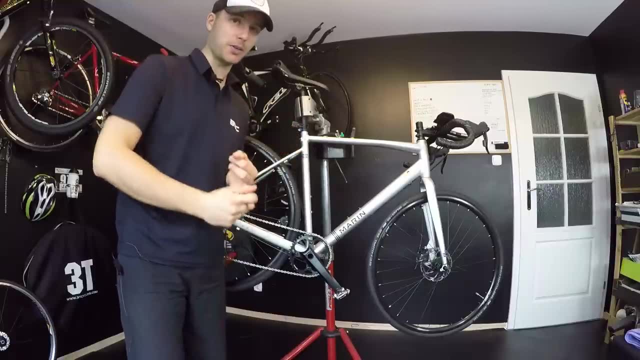 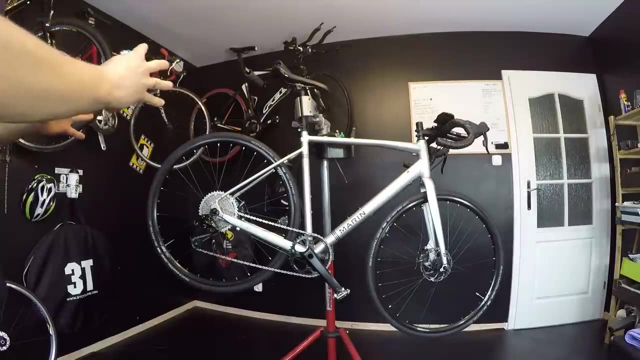 that some bolts are aren't just made or tightened well enough on, doesn't matter, either five hundred dollars bike or five thousand dollars bike, unfortunately, all right. so once we have done our wheels and tires and the bolts, then there comes the chain and i would say almost all of the 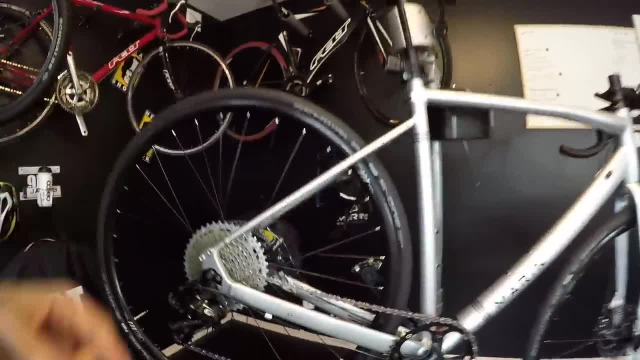 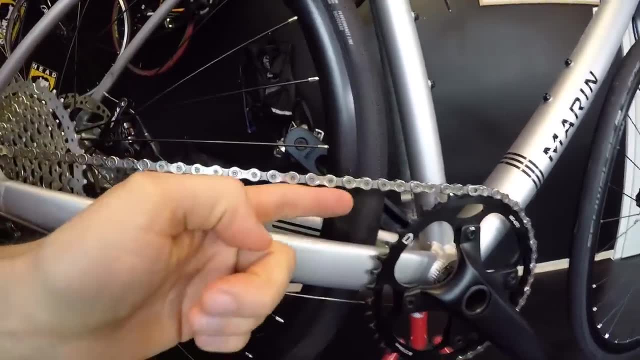 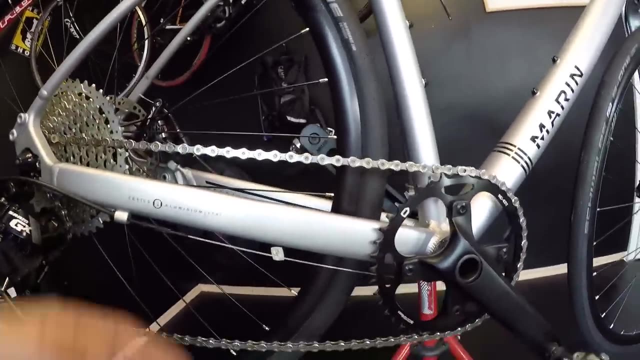 bike need this. first off, maybe make sure that you have the directional or undirectional chain. if the chain is directional, that means that it has the outer plates and the inner plates, and the outer plates should be on the outer side, of course. so if the chain has any signs on it, you 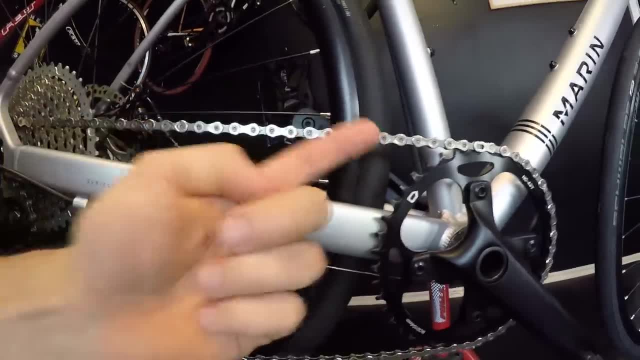 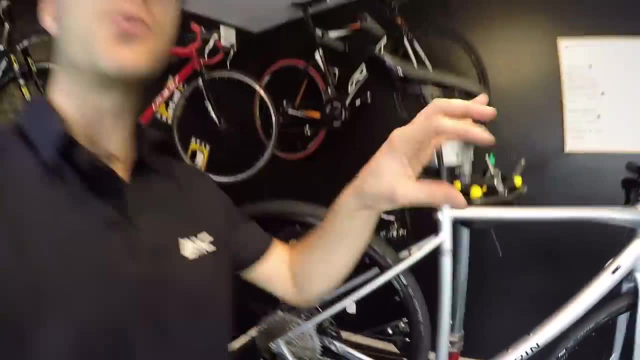 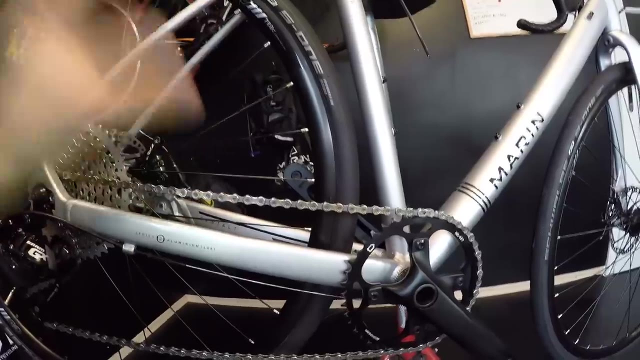 should see those on the outside. if it's just plain you don't see any like shimano hgx anything, that means it's been done in the wrong way, and that was also my experience with my canada brand new canada cat 10. so that's just a little thing you should remember about, but the huge part of the 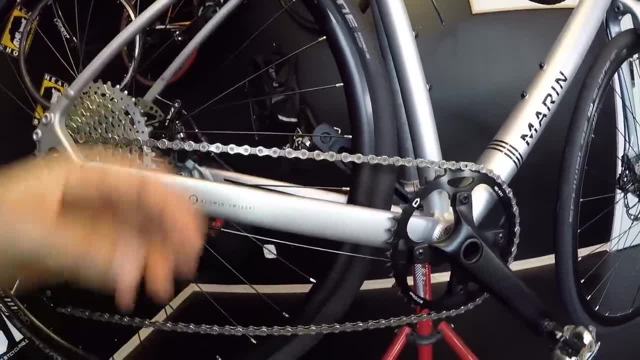 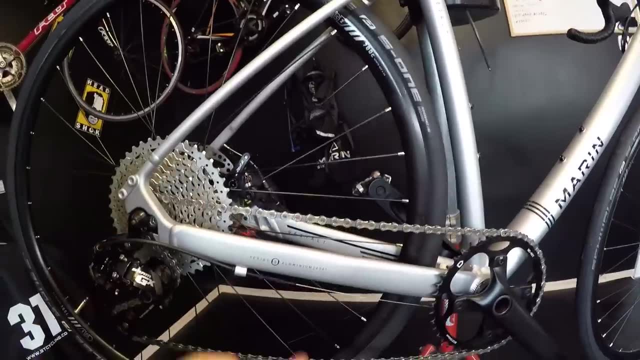 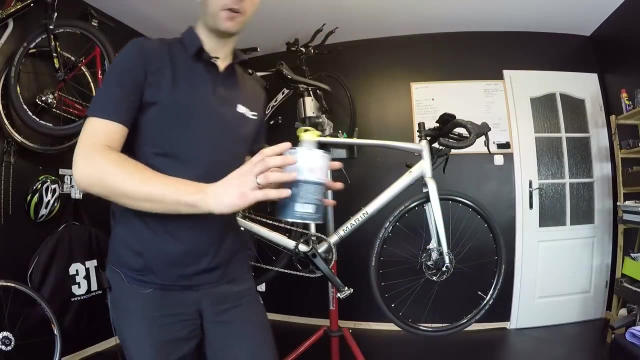 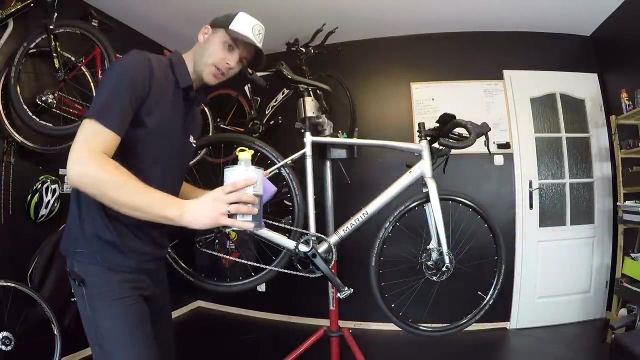 chain is that when you get the new bike with the new chain, it's so sticky. now there is one thing and the other which is don't, for this part. now, what this chain needs is it needs some kind of the degreaser and some cloth or wiper don't. here is something you should not do, is that you should? 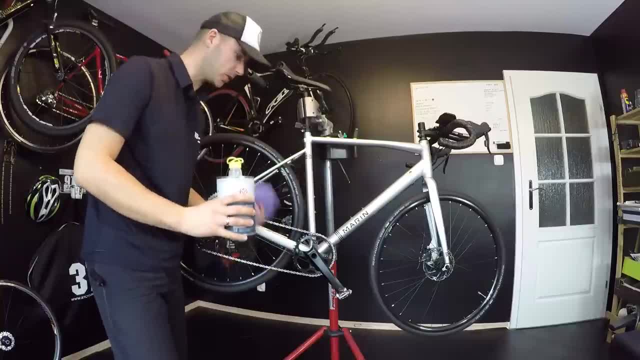 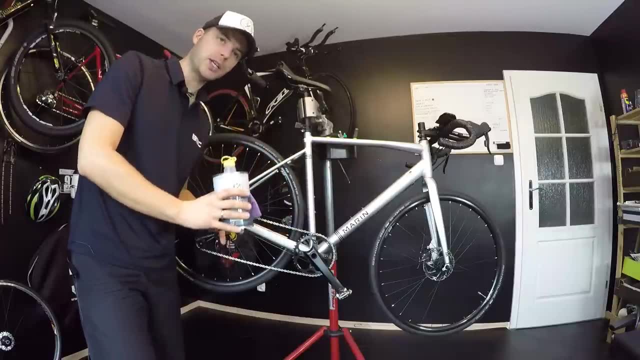 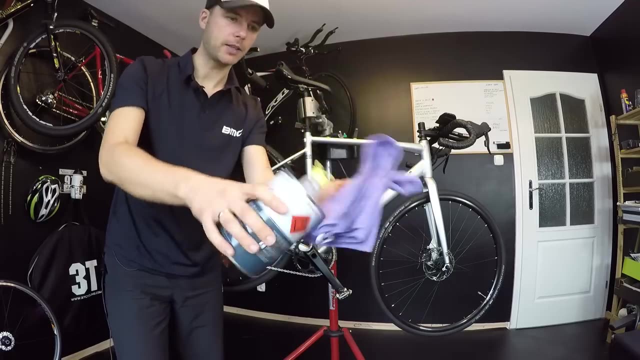 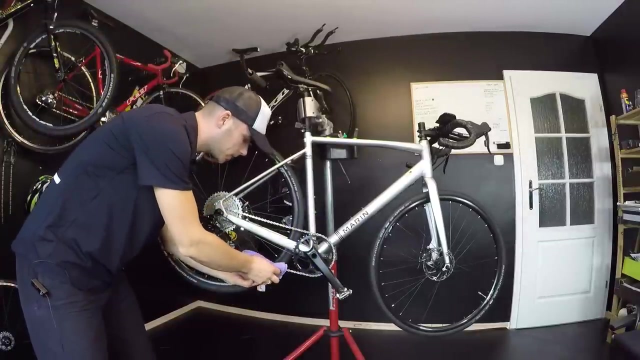 not dip your chain into the degreaser, because you need lubrication of your chain from the inside out and also it can damage your chain, actually, depending on what kind of degreaser you use. but if you simply do something like that with your cloth and then i'm just holding this cloth, 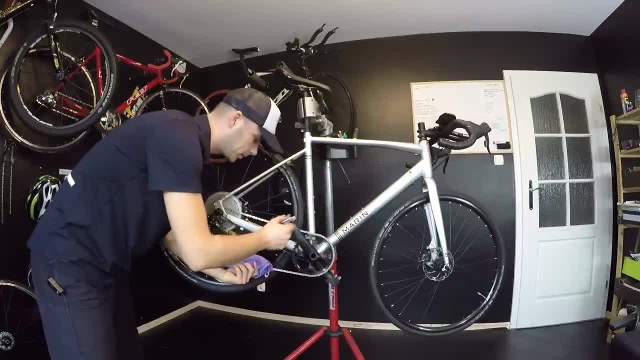 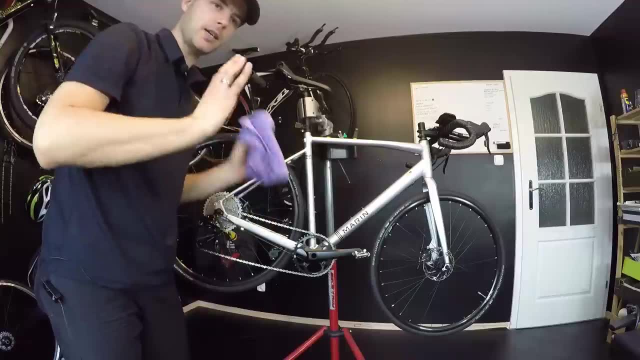 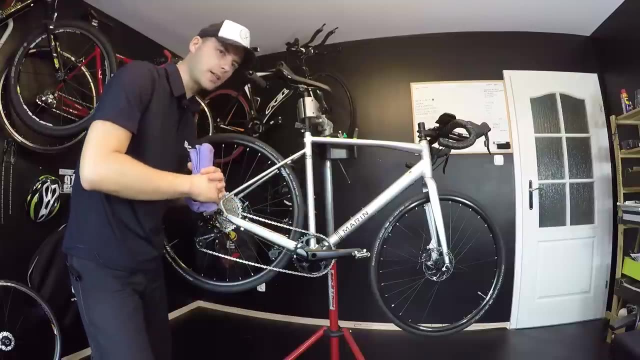 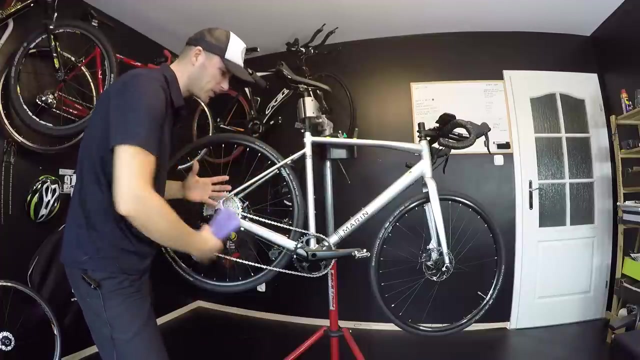 around around my chain and i pedal backwards for a couple of times until those plates from the from the outside are not so sticky, i'm done with my work. won't have to be lubricating your chain for a couple of rides because this original loop is sticky. so it maybe makes the drive train work bit harder, but it's okay. it will prolong the life of 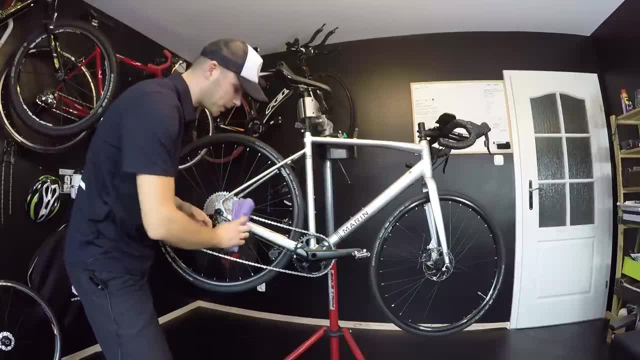 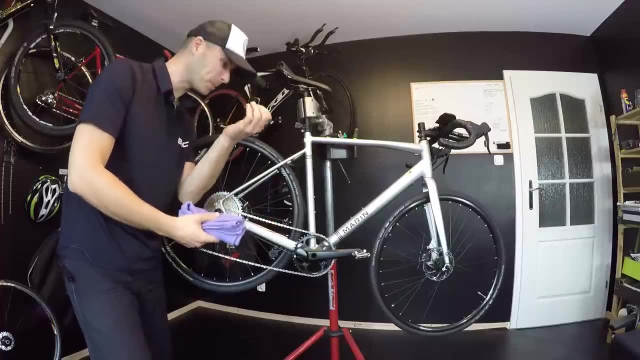 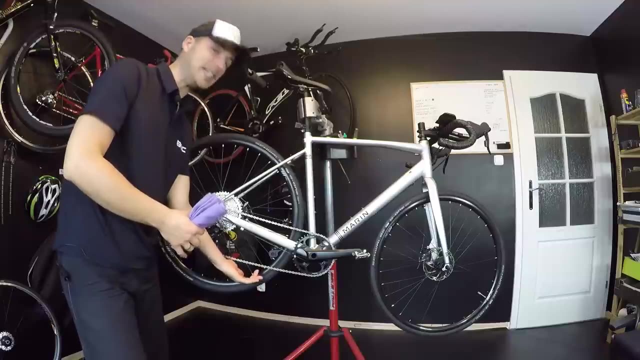 your, of your chain actually. but from the outside it should not be sticky. otherwise, if you just take your brand new bike with the brand new chain with this lubrication on it, it will be sticky and then you will actually have to deep clean your chain because it will be. 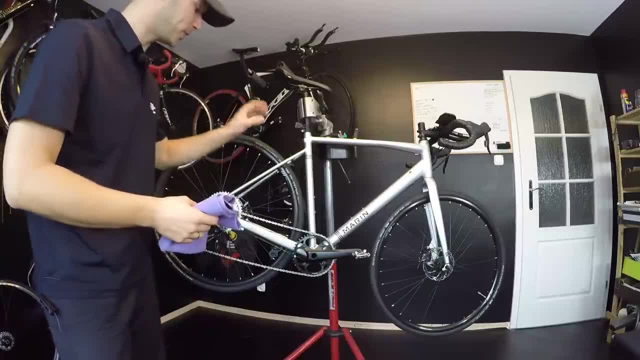 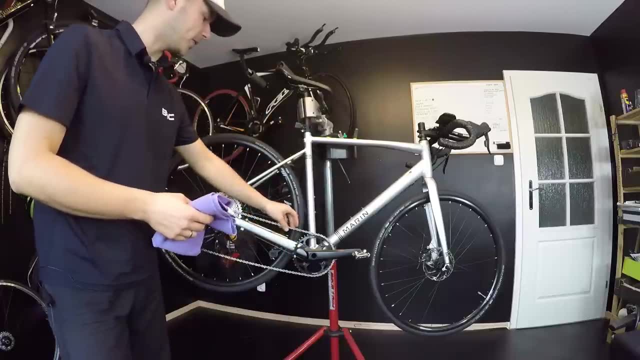 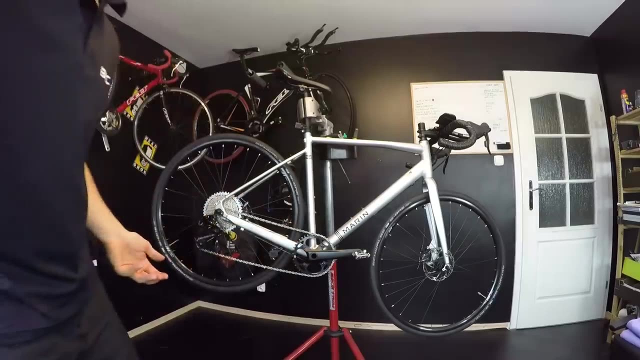 so, so dirty, all right. so we've checked whether the chain is being assembled in the right way. you should see the the logos on the outside. the chain is not sticky anymore now. the little part, but also so important for us, and it's the protection stickers- most of the bikes 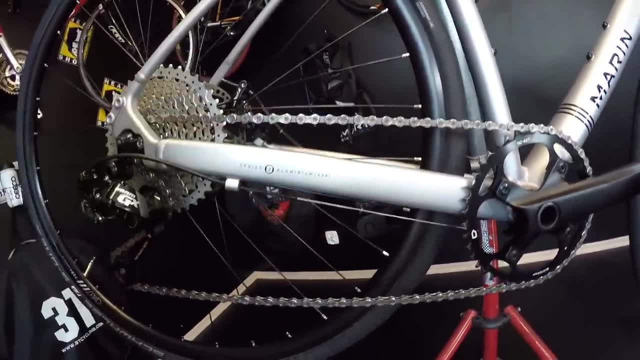 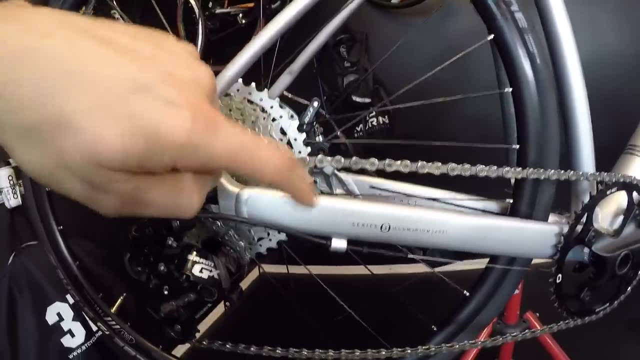 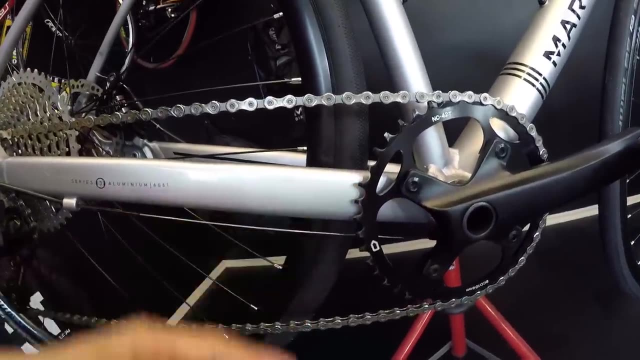 would have some small sticker here on the chainstay, which is way too small in my opinion, because you will be able to scratch your chainstays with the chain just behind it. as you can see, this sticker ends here. but, even more importantly, there is no protection here between the chainstay and the chainring, which 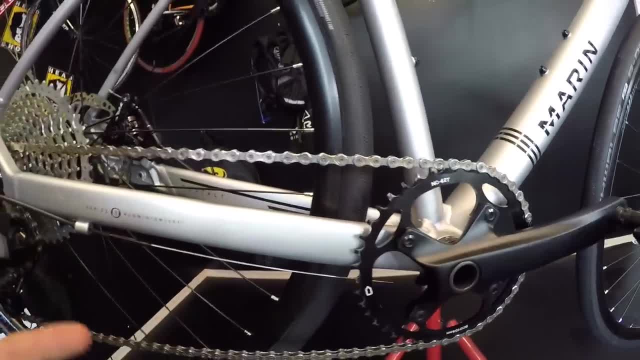 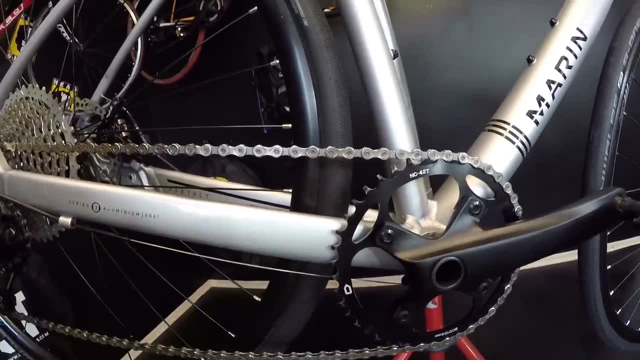 should just not be like that. of course, with the carbon bike it's even more crucial, because you can actually damage the carbon. but but here you don't want to have those, those nasty scratches. that's why you need some protection. i'm going to show you that in the 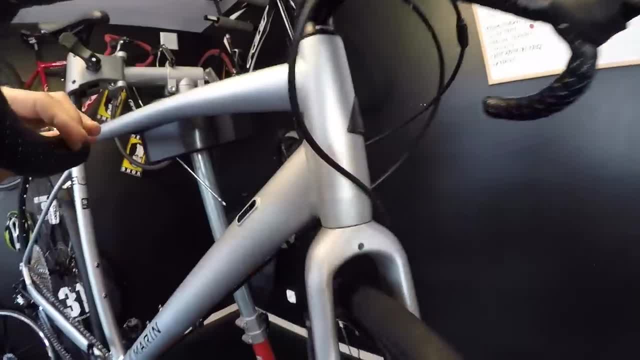 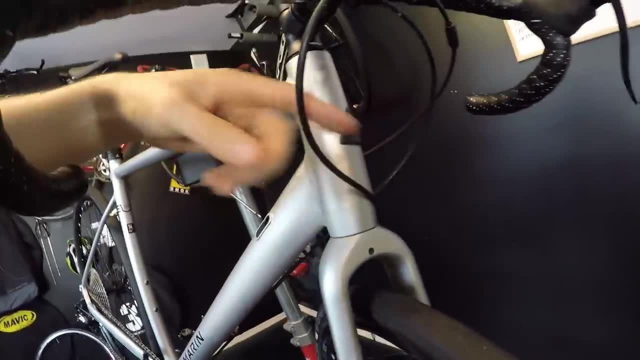 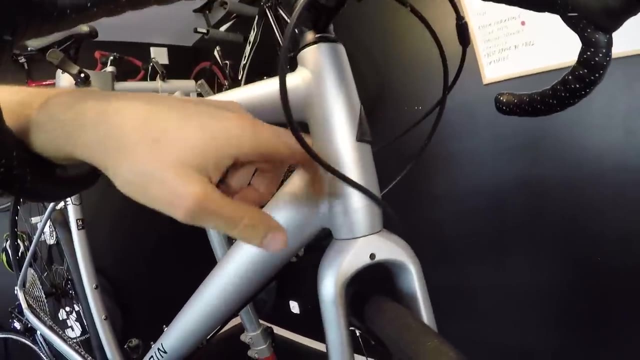 minute. but other place here is the head tube or actually anywhere where you have the housing rubbing against the the frame. as you can see, this front brake housing is beautifully rubbing our headset. if there would be any kind of dirt or mud, you will very quickly get rid of your beautiful. 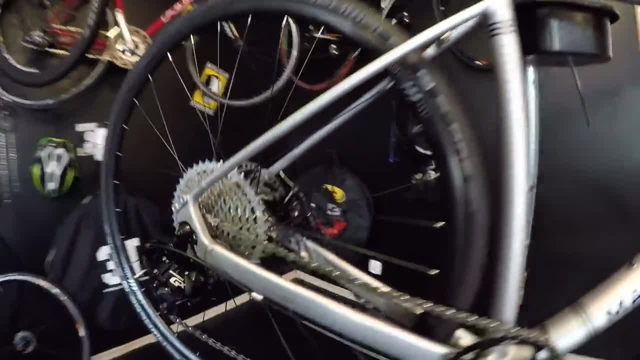 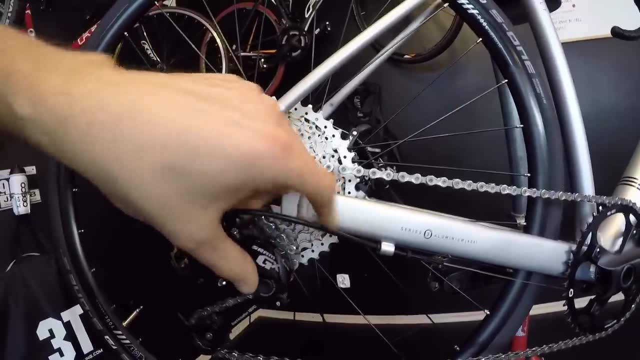 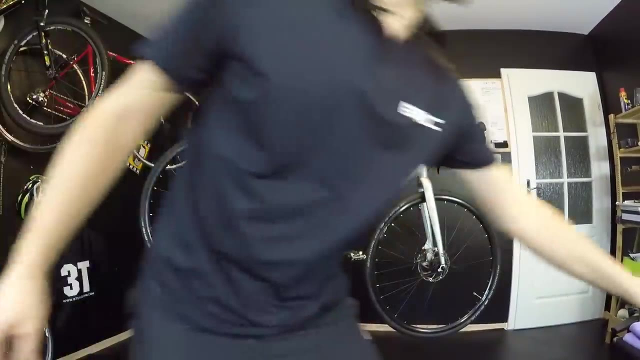 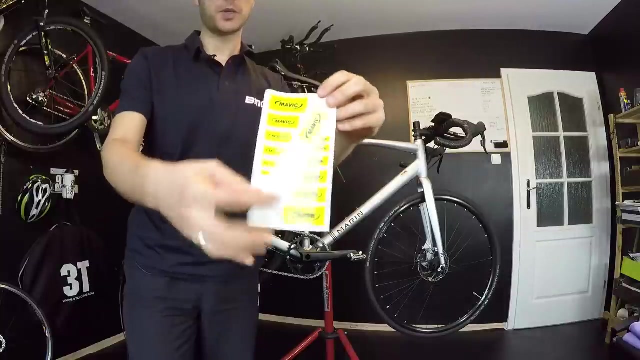 paint on your bike. so that's one thing. and also here in the rear, the last part of the housing to the rear derailleur will also just take off your paint from the, from the frame. so what you want to use is either some original stickers like protective stickers- these are from mavic and there is some special 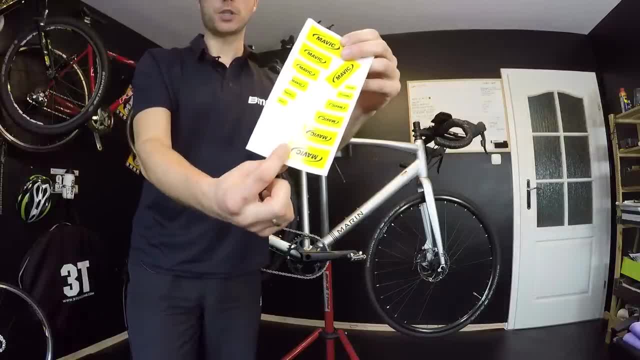 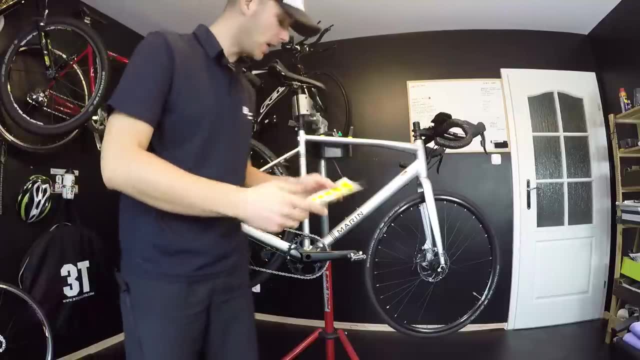 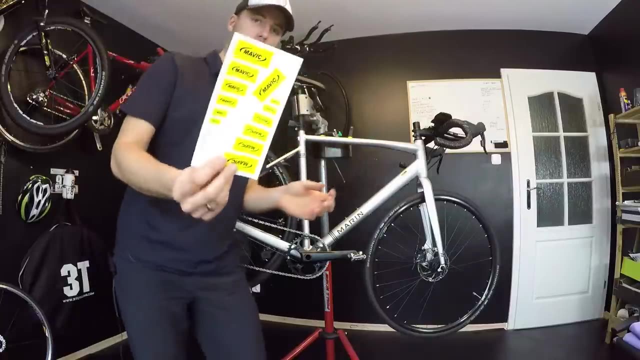 sticker for the chainstay and then different sizes of the stickers for your head tube, or also maybe between the housing of your rear derailleur and the chainstay, also between the chainrings and and the chainstay. so you- just you- can purchase this, this one and such thing and use it, but also 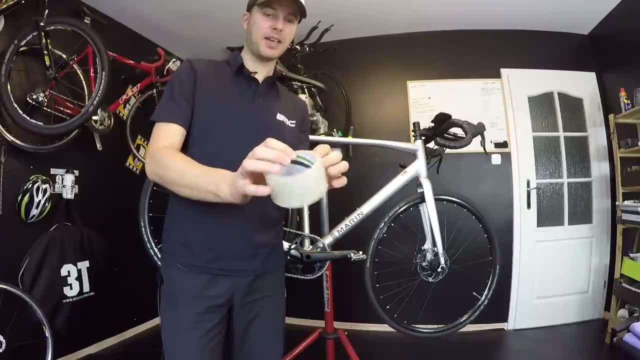 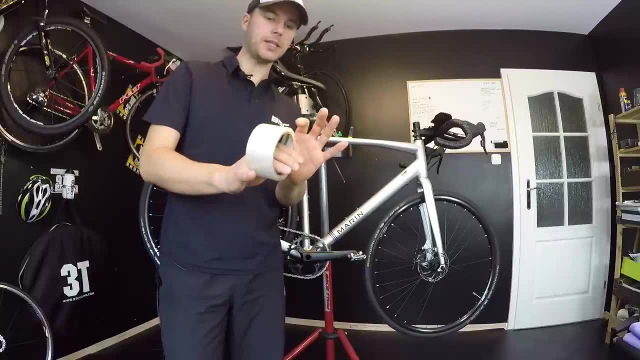 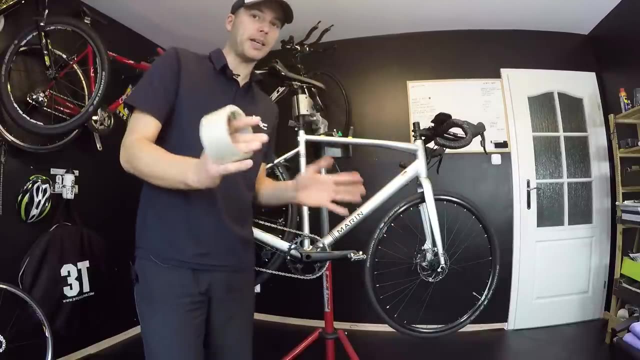 you may simply want to use a tape, and also you will be able to replace this periodically. now there is one thing you should be aware of, and it's what kind of a glue that the. the tape has perhaps damaged your paint on the bike. i don't know about that. this is just the example of the tape i've 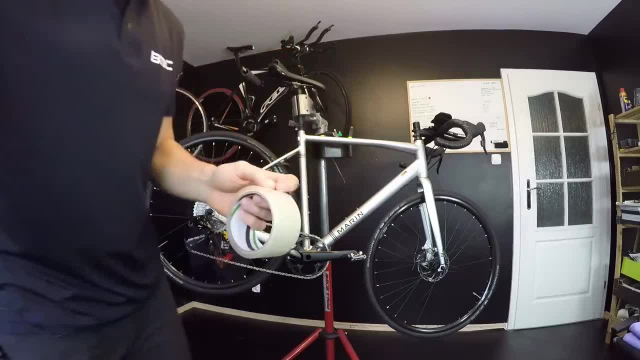 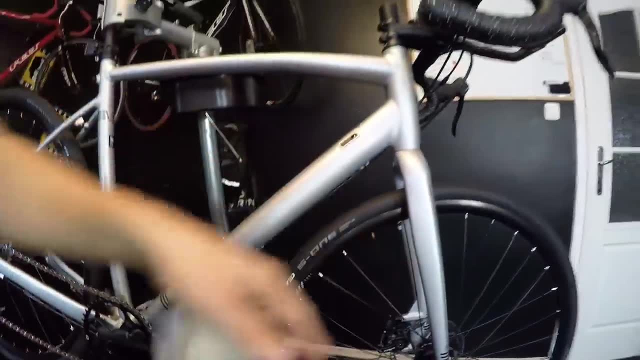 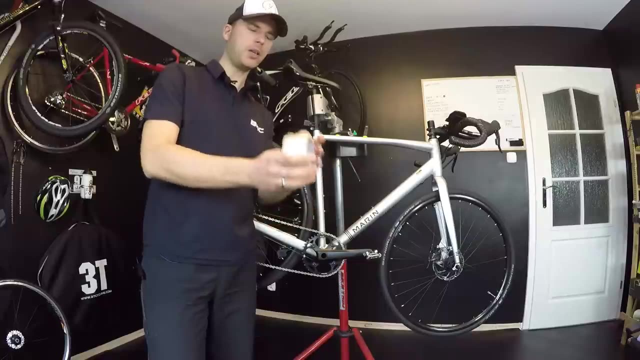 been using for years and i was using this one for some cadence sensor like under the cadence sensor and speed sensor on the bike, and i've never had any problems with with the paint and this tape. the only problem here is that if it stays on the frame like very, very long time- for maybe a year or- 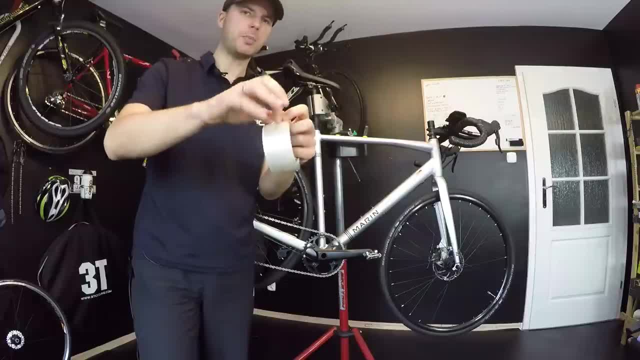 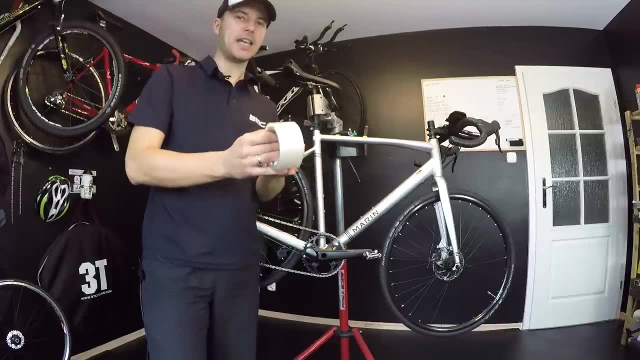 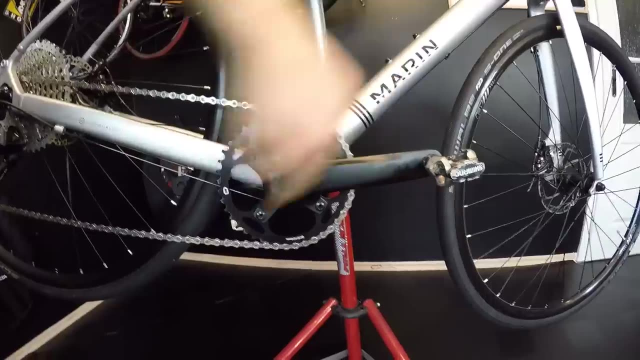 it will be more difficult to take it off because it will be just ripping apart, but it's just okay and then you can replace it. it stays clean and looks nice. of course there's there are also some special stickers designed for the crankset. it's nice to have this anodized crankset.